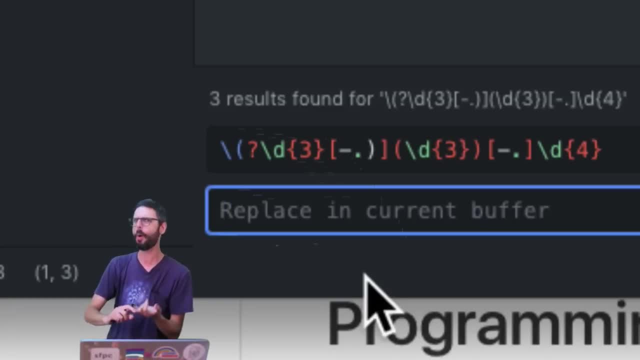 but they aren't inherently something that only has to do with JavaScript or Python or Perl or Java or C++ or even programming whatsoever, and, in fact, a lot of what I'm going to show you today is how to use regular expressions just as a tool for 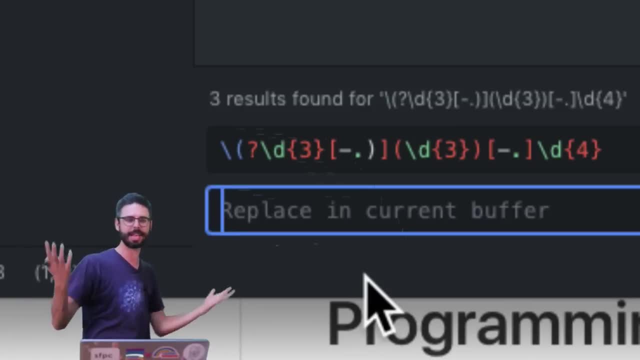 yourself in a text editor for writing or find and replace and that sort of thing, And you can see. so here's the downside of regular expressions. The downside of regular expressions is that's what they look like, So they're possibly one of the most cryptic, strange-looking things that you could ever possibly create with. 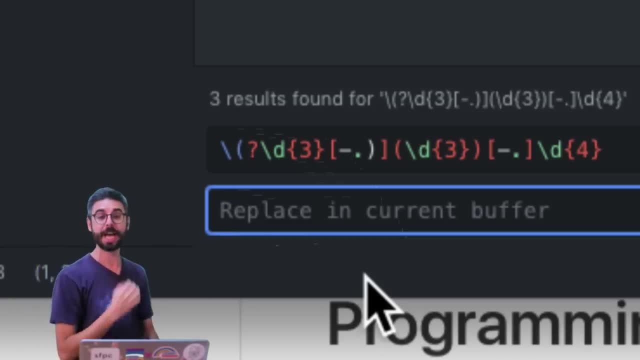 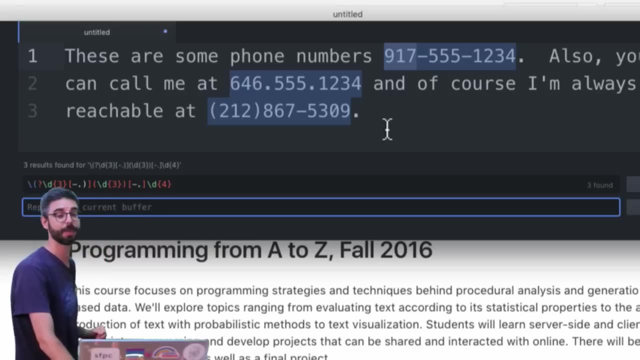 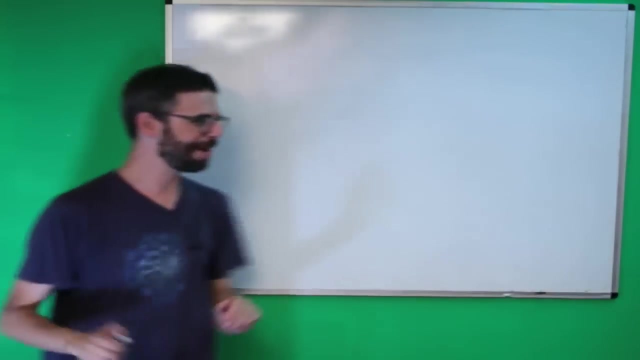 strings of characters, And this is in fact a regular expression that is searching for phone numbers, and you can see here that magical regular expression has found these three phone numbers in this particular piece of text, which leads me to the discussion of what a regular expression actually is. I don't know why. 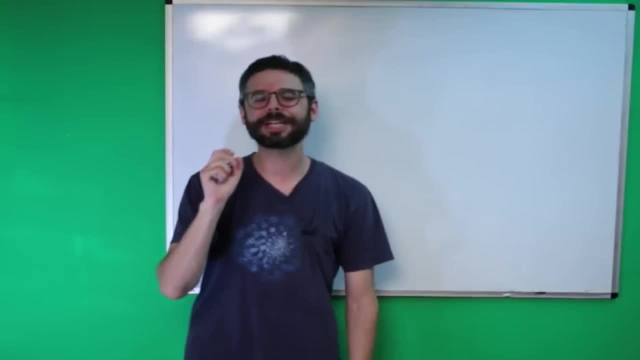 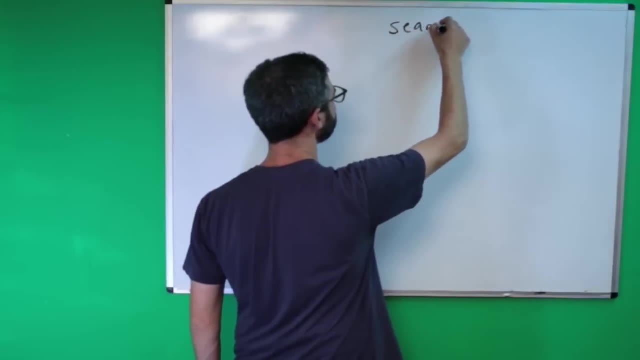 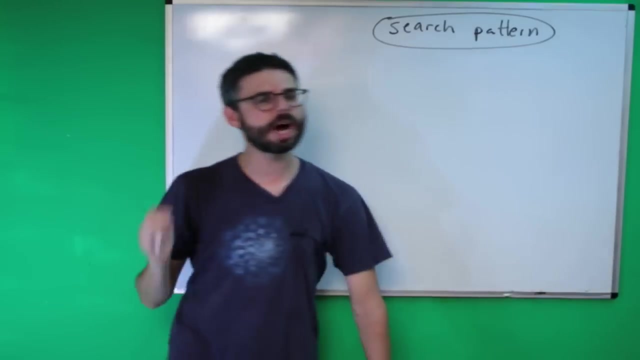 I'm coming over here, but I am Okay. a regular expression is a sequence of characters that defines a search pattern In a search pattern for text. so it actually comes, you know, if you look at the history of why these regular expression things exist. read about this. 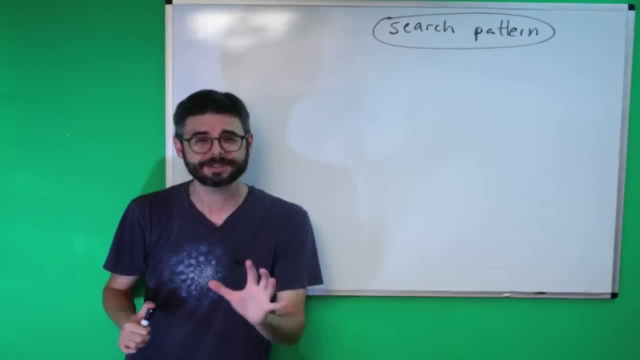 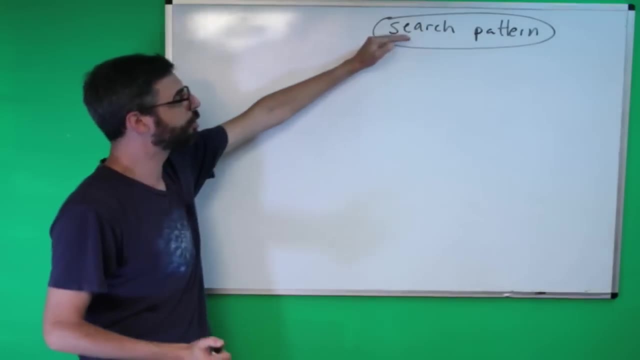 on Wikipedia, you'll find that it comes from the mathematical concept of regular sets, sort of an interesting side note. but here really what? what I want to show you how to use them is how to define a search pattern in a body of text. So let's, let's talk about what this means exactly. 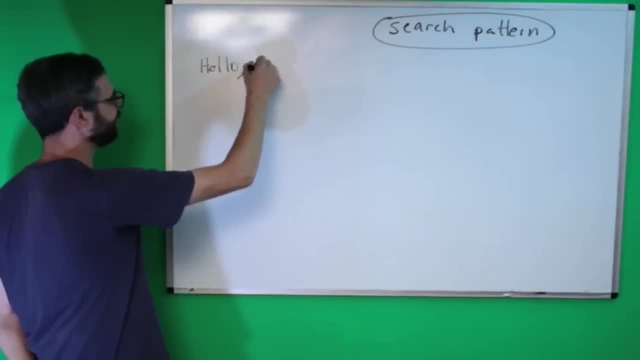 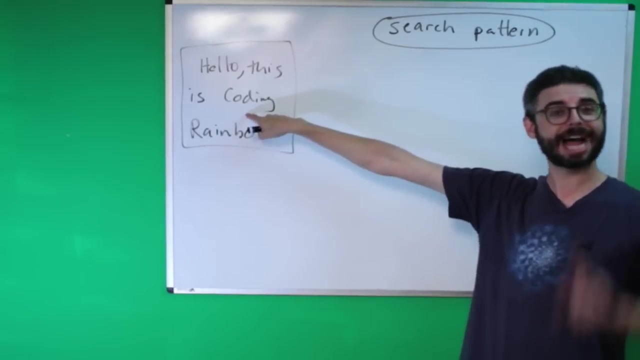 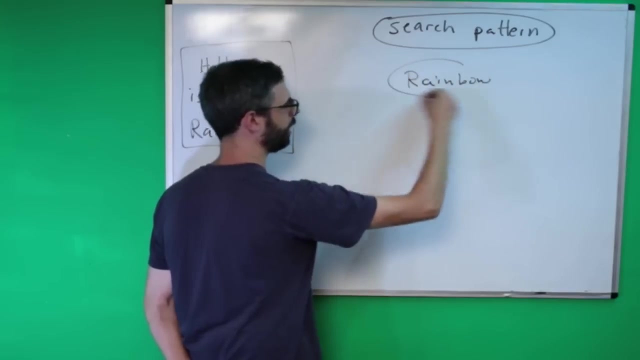 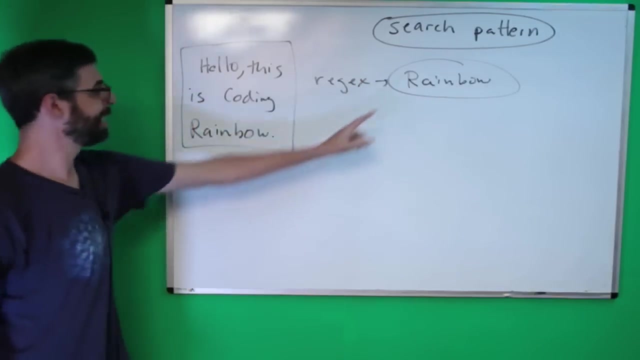 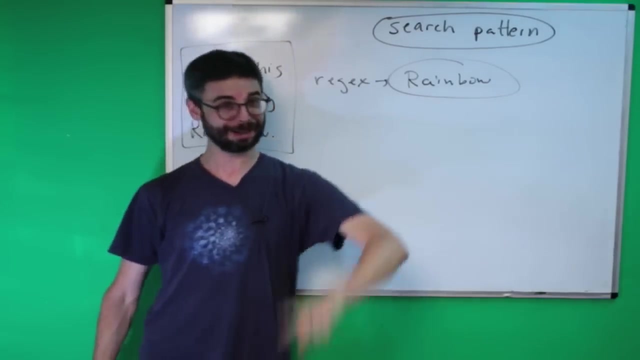 Hello, this is Coding Rainbow. right here is text. okay, now I want to define a search pattern to search inside this text. here is a regular expression, often referred to as regex, for short regular expression. this is a valid regular expression. it is a pattern. The pattern is as follows: capital R followed by lowercase a followed by 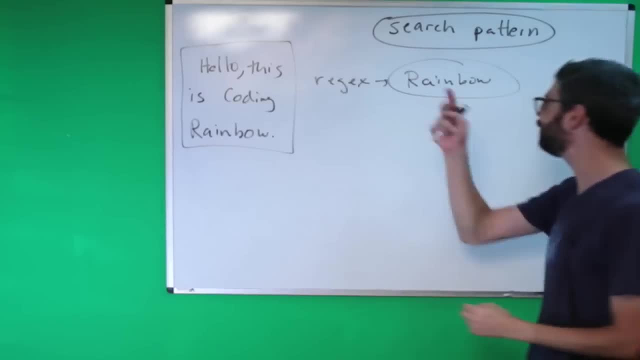 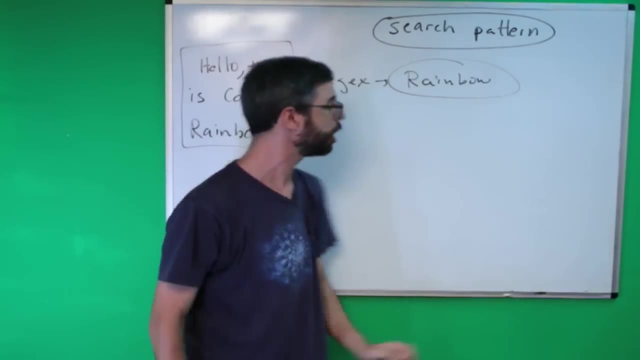 lowercase i, followed by lowercase n, followed by lowercase b, followed by lowercase o, followed by lowercase w, and you might think it absurd that I went through that whole thing, but this is exactly how you need to think of regular expressions. You need to look at that sequence of characters and translate. 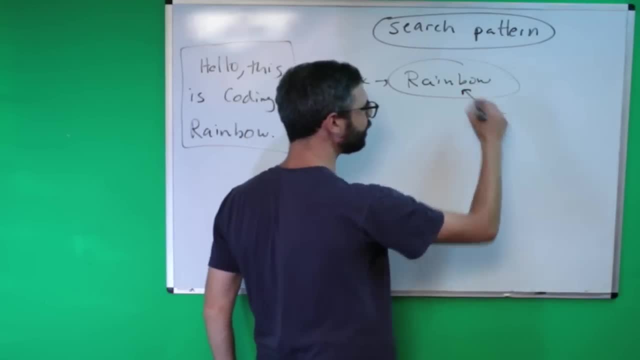 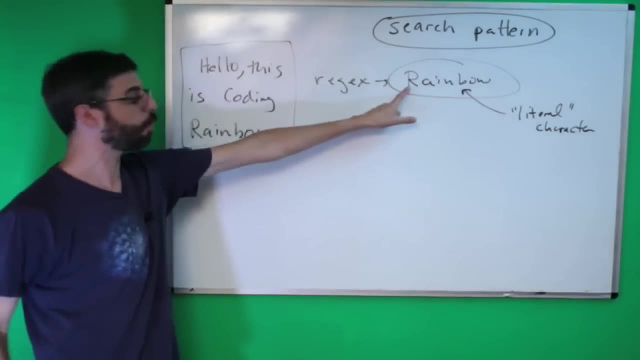 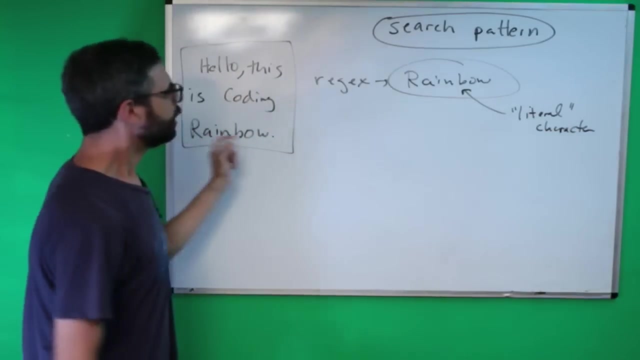 what each character means, and in this case, each one of these characters is what's known as a literal character, meaning the pattern is. the pattern that I'm searching for is literally the character capital R, followed by literally the lowercase a, so you can imagine what would happen if I go over. 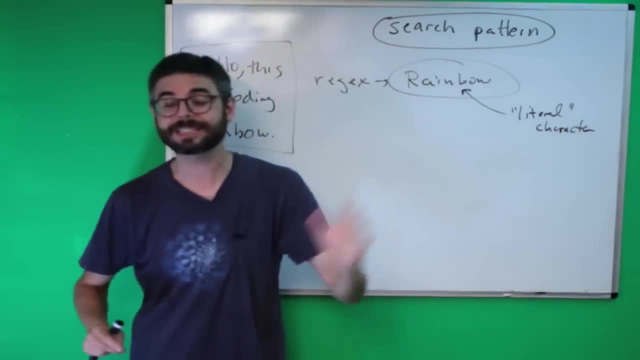 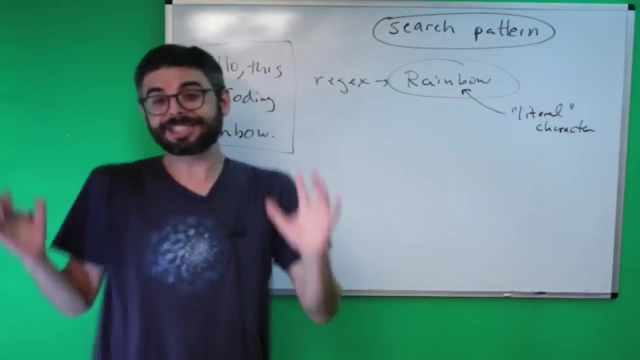 to. I'm not going to go over there. if I go over to text editor, I hit command F, I'm searching in the text. I type in rainbow. it'll highlight for me every time rainbow appears. Now this is unto itself not super powerful, yet when you 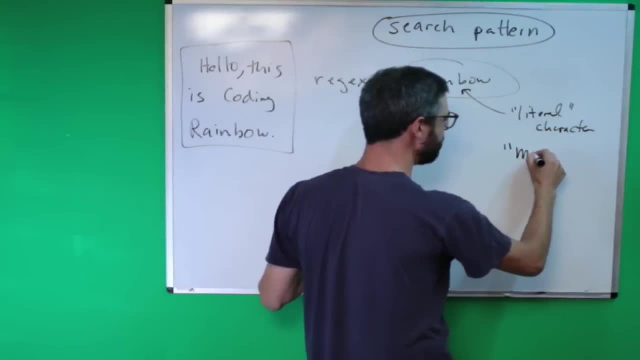 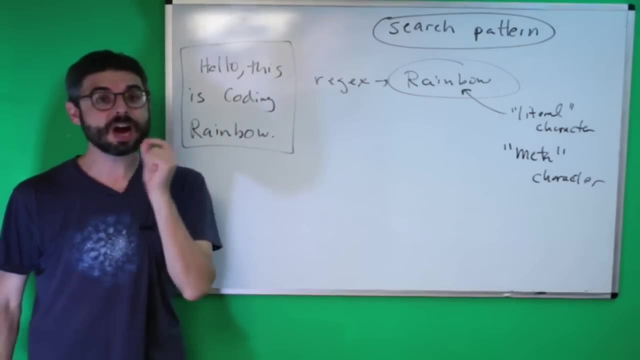 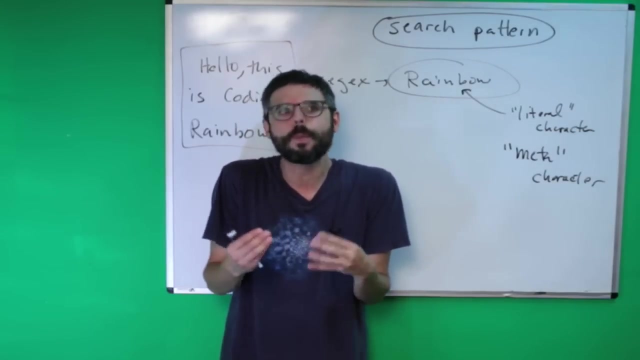 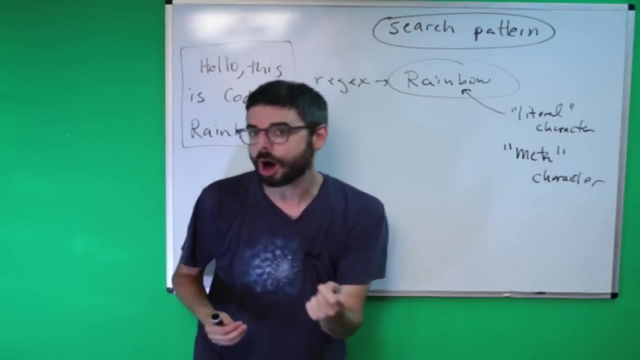 add the addition of this idea of something called a meta character, a meta character meaning a character that does not indicate a single literal character, but a character that indicates some type of more generalized pattern. for example, I could say: I want to match the capital letter R, followed by any. 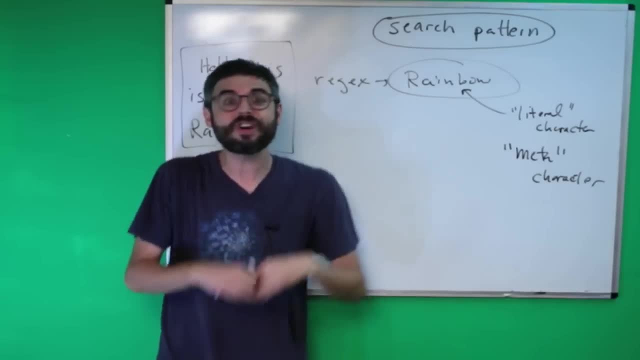 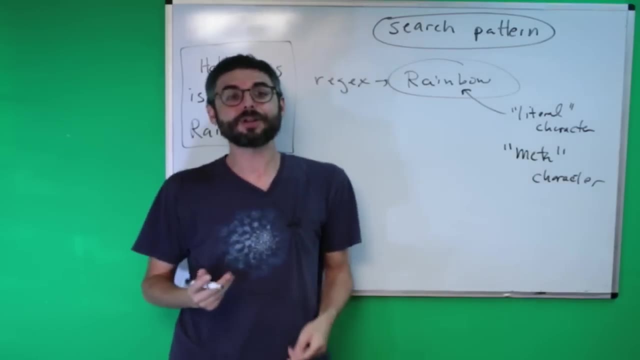 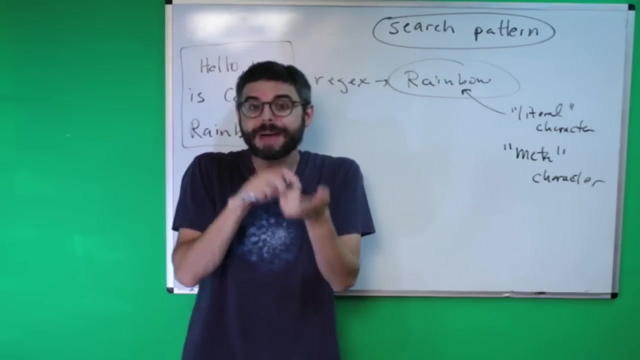 possible vowel, followed by the any possible vowel, followed by any possible consonant, followed by any possible uppercase character, followed by any digit, followed by any white space. you can imagine how you can start to create more and more generic patterns that were multiple, that would match different kinds of text. so let's think about this a little bit more. I'm going to come back. 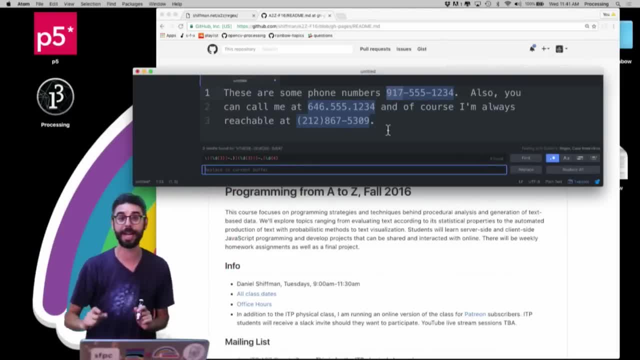 over here for a second and point out. let's think about the phone number example. I think it's a useful example to start with. imagine you had a huge text. you've got access to this massive text and you want to publish it, but it has lots of private phone numbers. 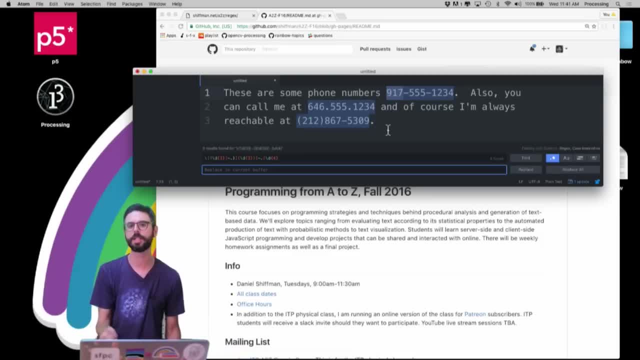 in it, and so what you ultimately want to do is redact the phone numbers. so you need a way of searching throughout the text for every phone number. but you can't say literally: I want to search for, not the actual numbers. you have to say I want to search for something like: I want to search for three numbers followed by 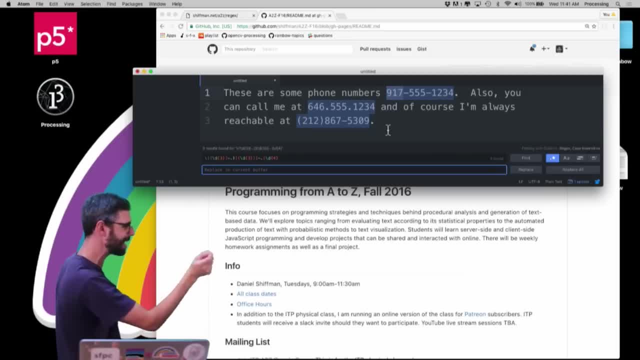 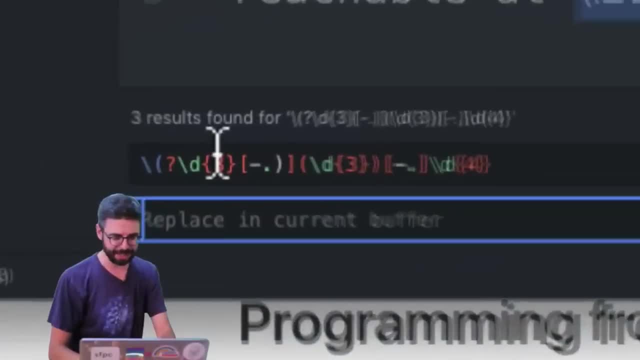 either a dash or a dot, followed by three numbers, followed by either a dash or a dot, followed by four numbers. oh, and it's possible, the first three numbers could have parentheses around them, and this, by the way, is exactly what this particular regular expression is doing. so let's go back and unpack this a. 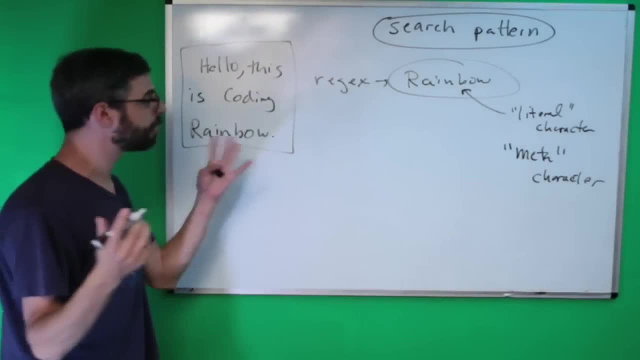 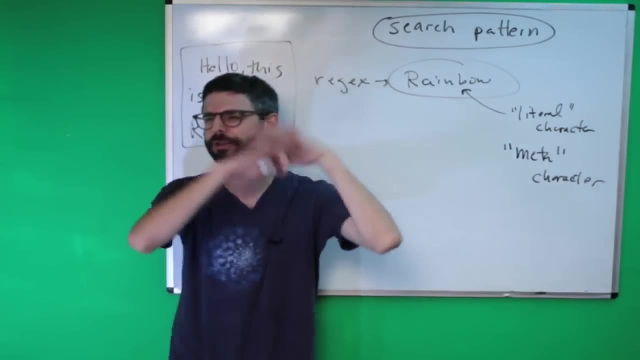 little bit more and let me show you what, what, some, what some meta characters are. so I want to keep a running list of meta characters and I think I'm just kind of in this video I'm just sort of introducing the topic and I'm going to. 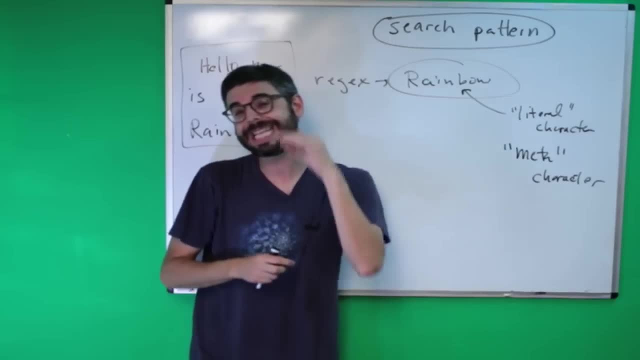 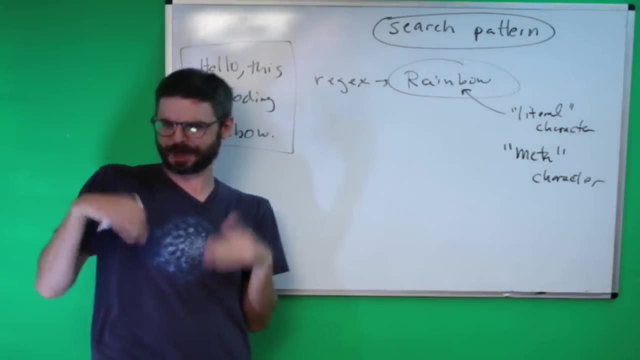 talk about this phone number example, and in the next video I'm going to kind of start to go through the pieces of regular expressions a little more one-by-one, so I might jump around a little bit here. then I'm going to go through them one by one. I think that's going to work okay. 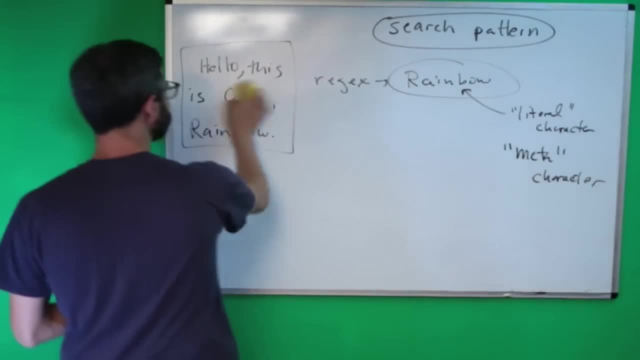 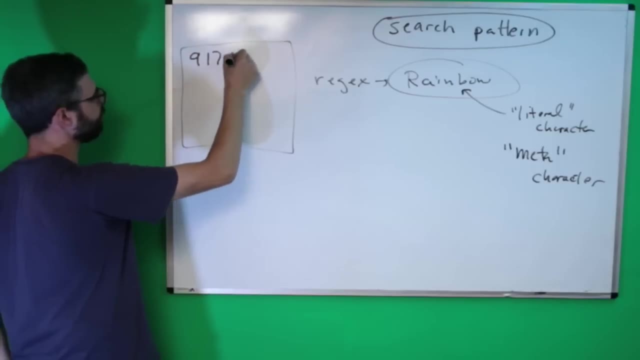 so let's think about the phone number example. so I might. the text that I'm looking in has this in it: nine one, seven, five, five, five, one, two, three, four and six, four, six, dot. eight, six, seven, five, three, oh, nine, okay, so how do I? I want to. 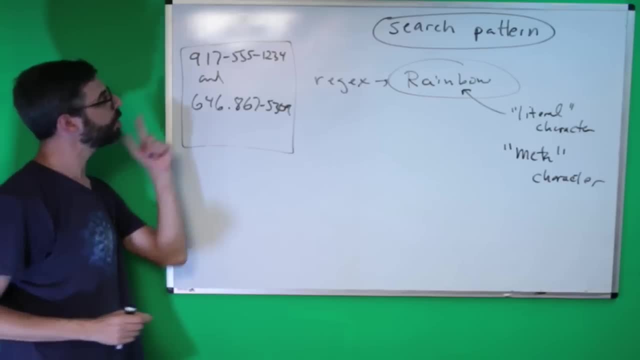 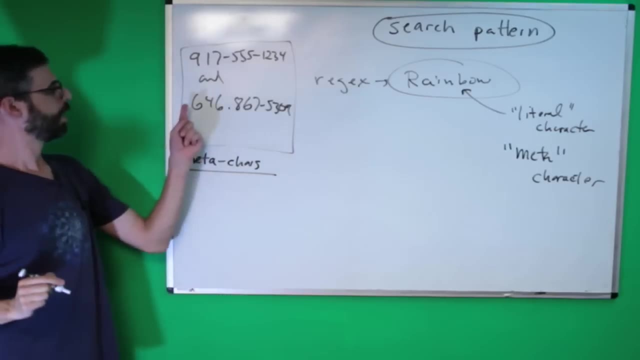 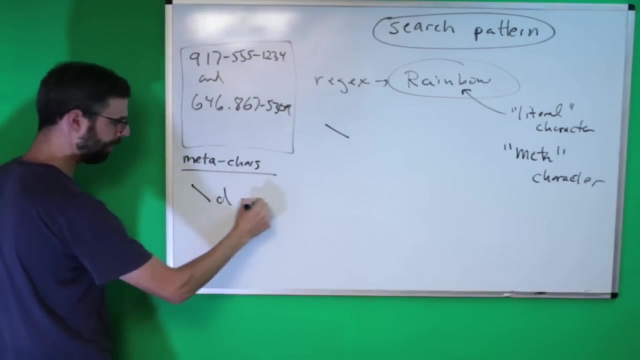 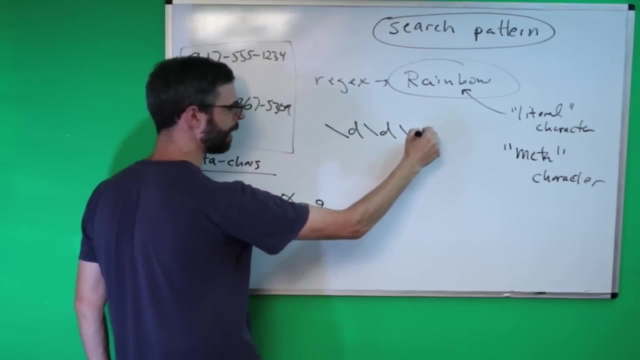 create now a pattern that will match these. so what could I say? and let's make a list of meta characters over here. the first thing I want to match is any digit. so guess what? backslash. backslash D means any digit, 0 through 9. backslash D, followed by backslash D, followed by 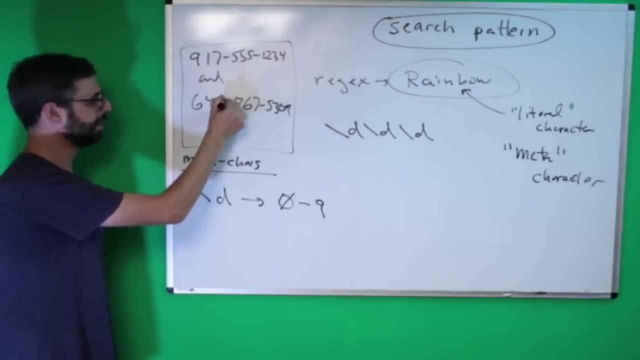 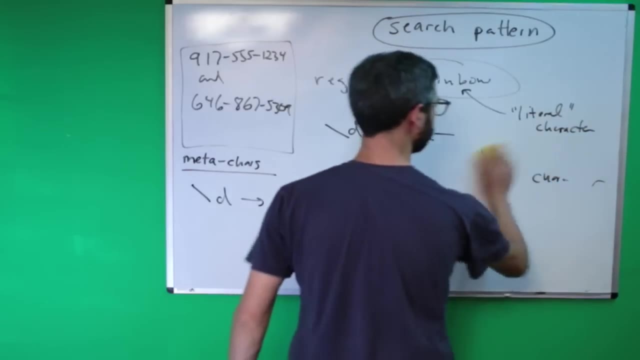 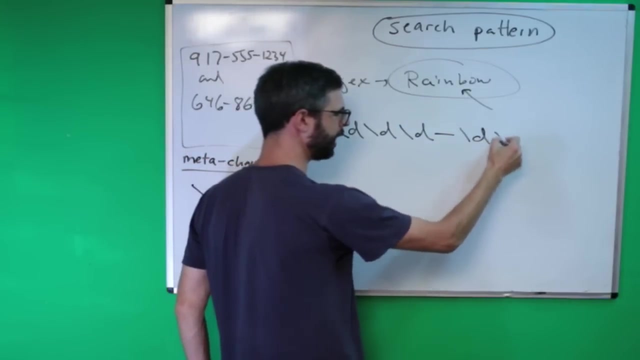 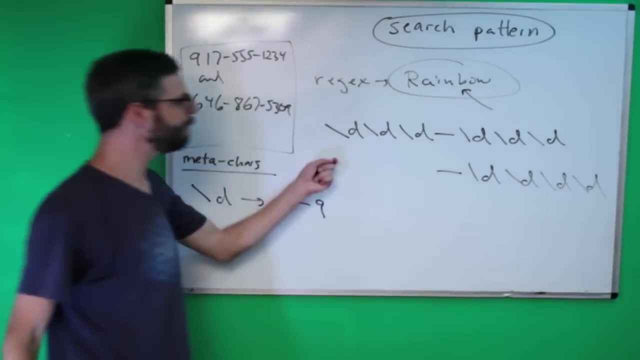 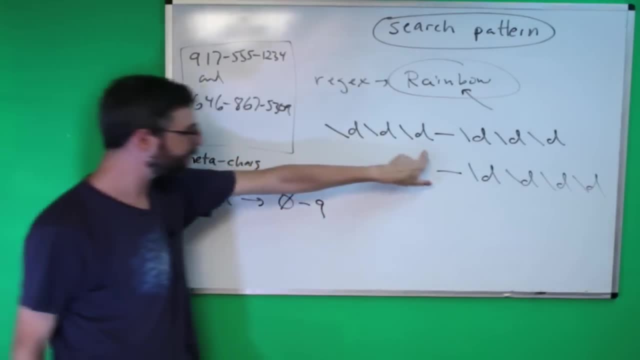 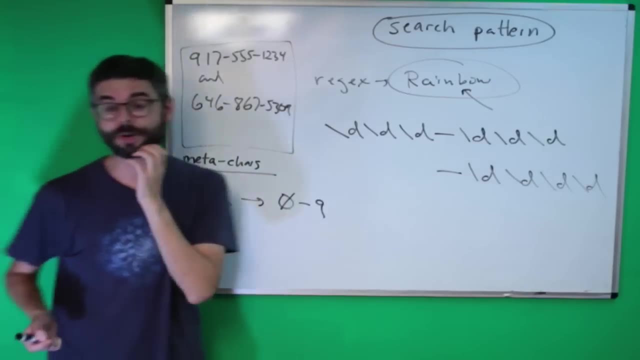 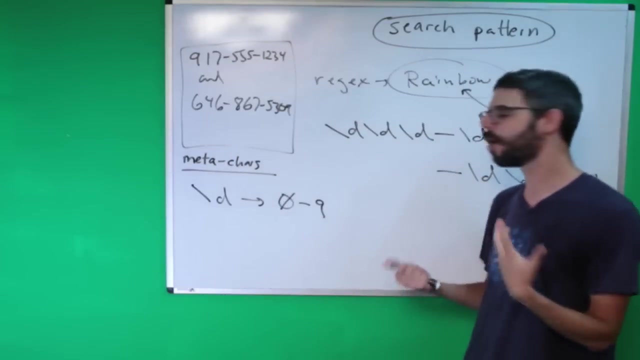 search for any text that matches three digits, followed by a dash, followed by three digits, followed by a dash, followed by four digits. so now what I want to do is actually show you this running in the wild, so one of the things you can do in most text editors. so, for example, the Adam text. 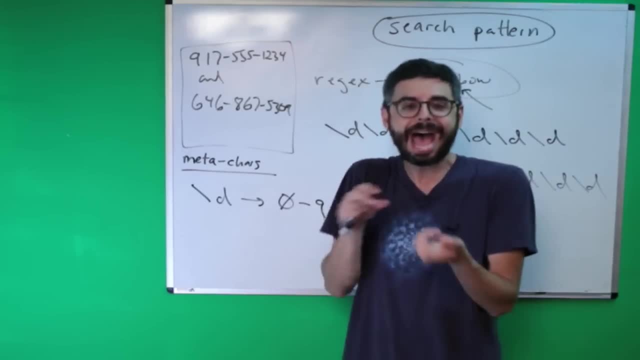 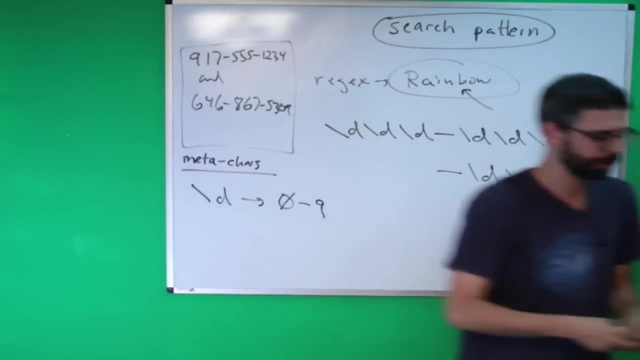 editor, the sublime text editor, a lot of things, tools that you might use have. when you do the command F for find, there's often a little button there that allows you to search by regular expression. so let's look at that. so I'm going to come back over here and I'm going to delete this. we'll make this. 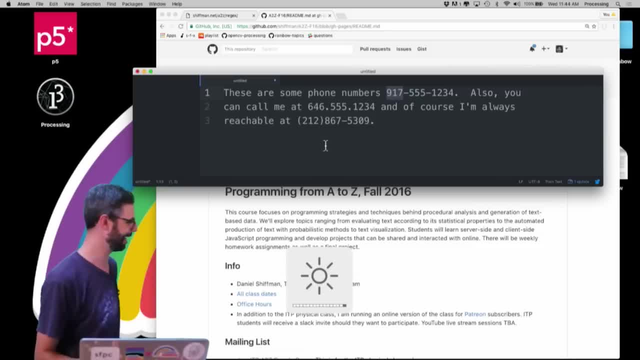 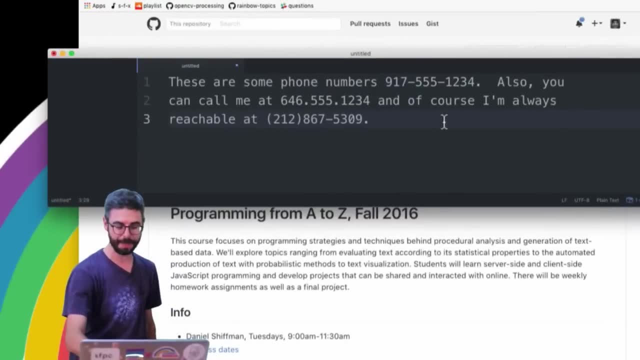 happen later. I'm going to do this, so pretend I'm like this. pretend I'm like this, I am like this. pretend that that other stuff didn't exist a moment ago. and now what I'm going to do is do command F, so normally I might do. 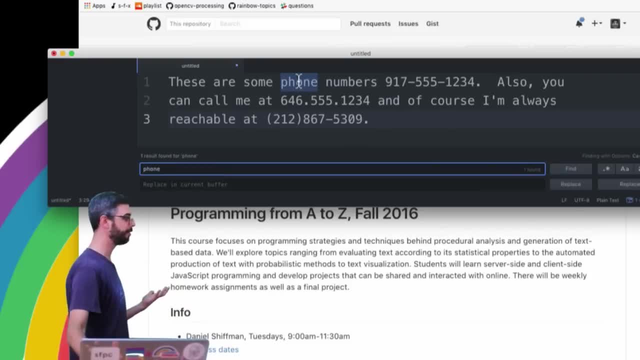 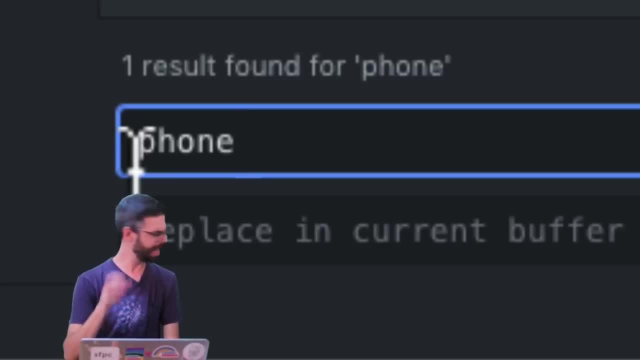 something like this: okay, type in phone and you can see it. highlighted phone for me. and I realize this text down here is a very, very small. I'm going to try to zoom into it when I remember, but it's. it's a Adam, doesn't? I can't seem to. 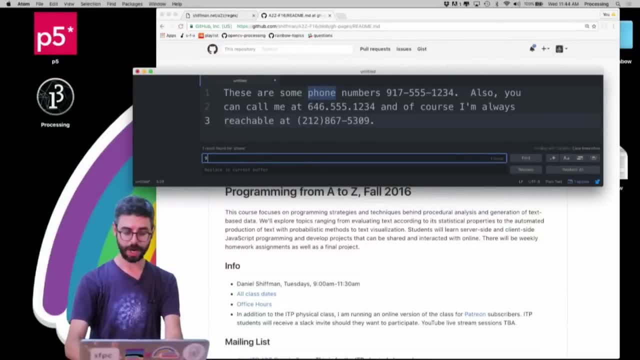 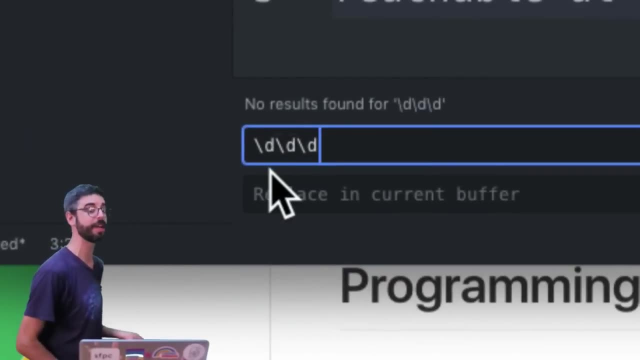 figure out a way to make that text bigger so I could also search for nine, one, seven, dash, five, five, five, and you can see I'm searching literally for this particular phone number. now what I said is I could do slash D, slash D, slash D. now look at this notice. this just looks like this is actually looking for literally. 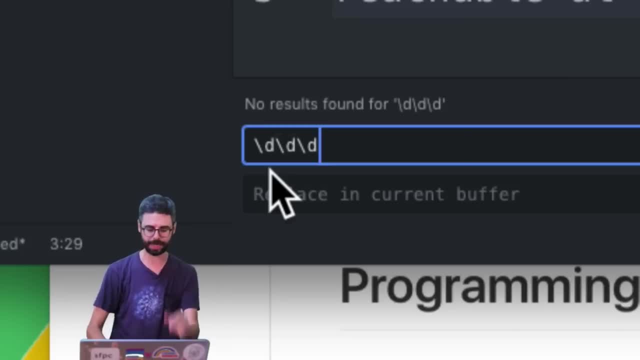 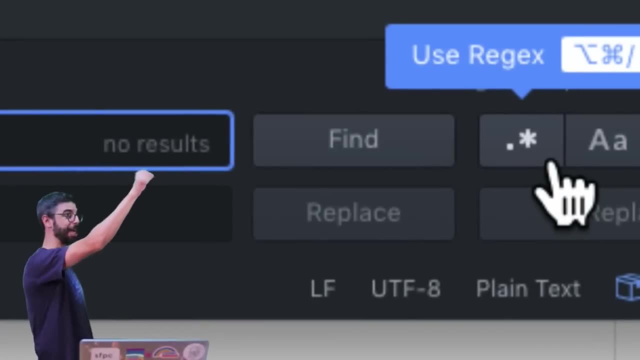 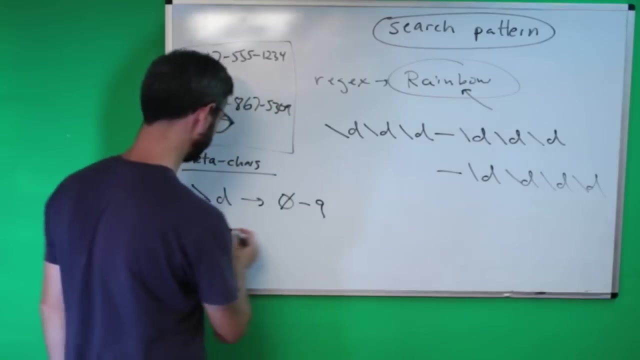 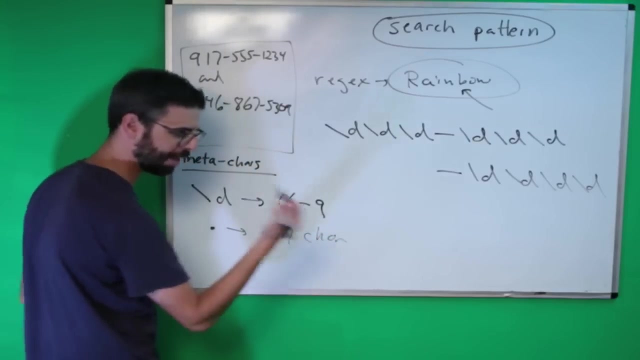 slash D, slash D, slash D. in order to enable regular expressions. I need to go all the way over here. see this button and it says use rejects. so that button enables regular expressions in the search. and incidentally, why is it dot star? so two more meta characters. dot means any character. I've got the wrong. 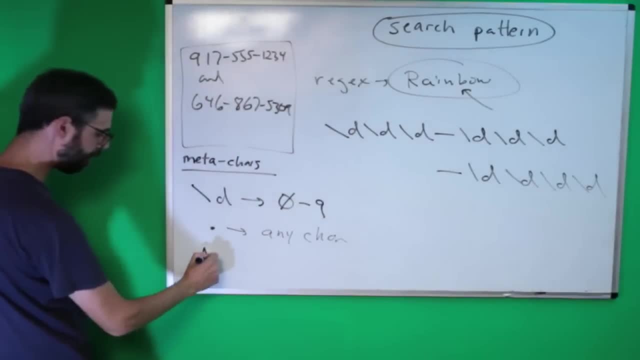 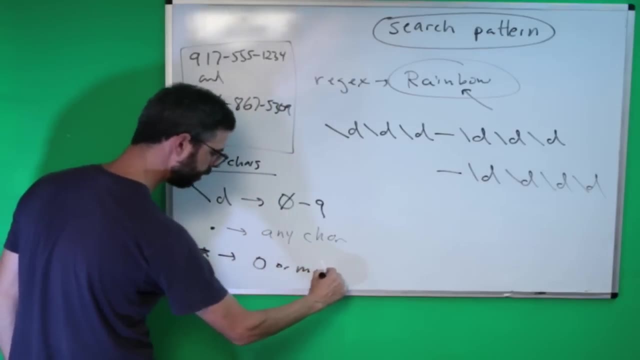 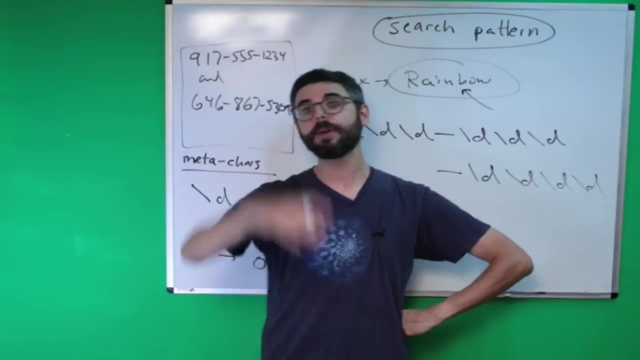 whiteboard marker again, and star is what's known as a quantifier, and again I'm going to go through this stuff in sequence, meaning zero or more. so this dot star which you've probably seen- like- oh, I want to look for all of my files- called rainbow dot star, that means it. 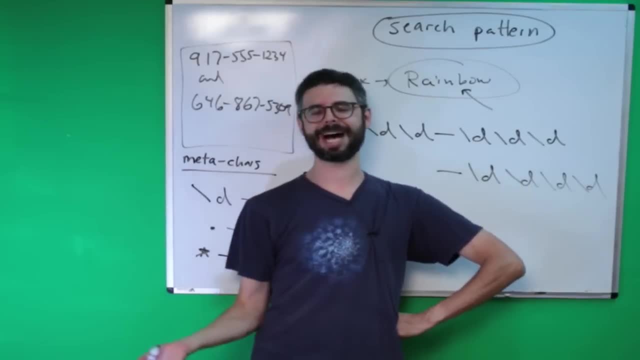 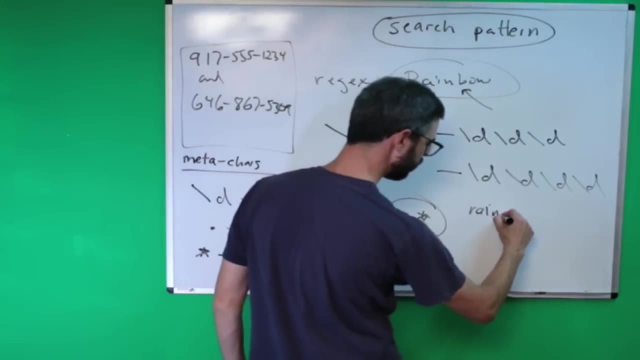 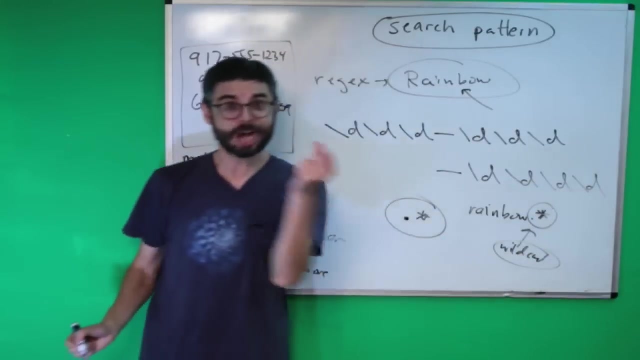 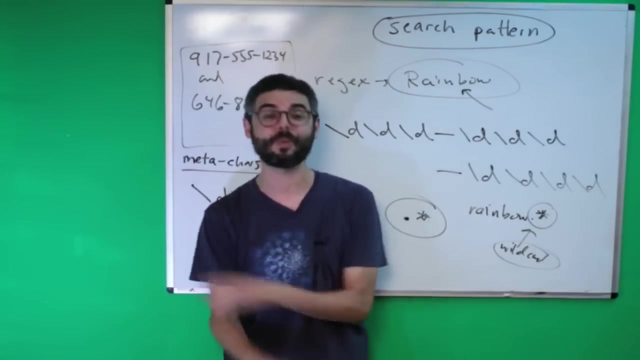 could be: rainbow cat dot PNG. or rainbow happiness dot JPG, or rainbow essay dot DOC. right any file right. rainbow dot star. this is often referred to as a wildcard and it is, in fact. it comes from regular expressions. this is a regular expression. it means I want to match rainbow, followed by any number of any characters- wildcard. 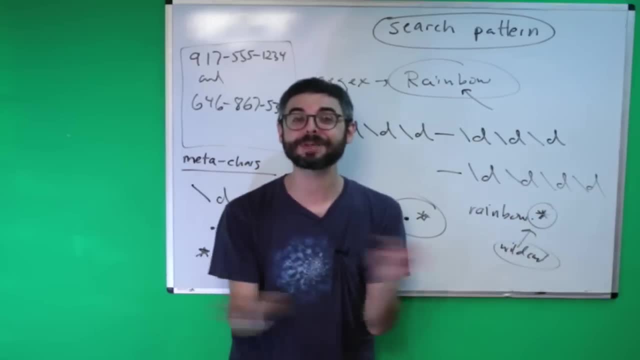 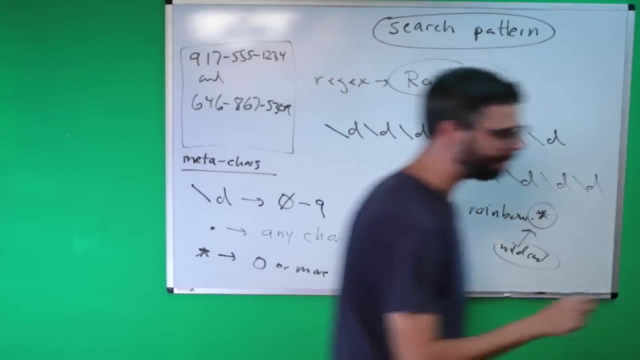 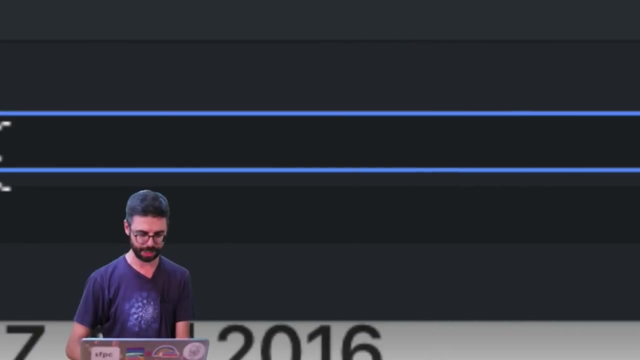 anything, zero or more anything. this matches absolutely everything in the known universe. this regular expression matches the universe. okay, so that's where that comes from. back over to here. we can see here dot star. so now I'm using regular expressions. as soon as I do that and I come back over here, can I?